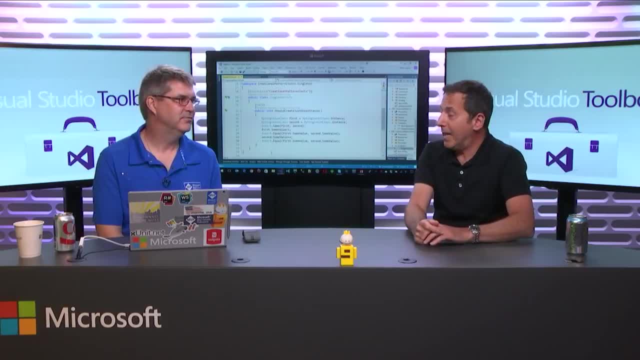 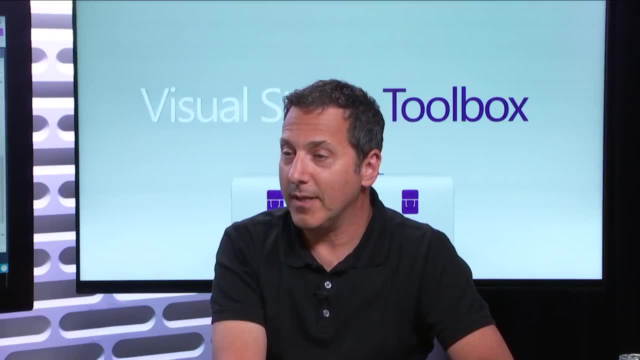 We are, And in the previous episodes we covered the behavioral patterns, We did, And we are now going to talk about the- Creational, Creational patterns. Yes, So let's just review the difference between the two. Sure, And it just occurred to me, we probably should have done. 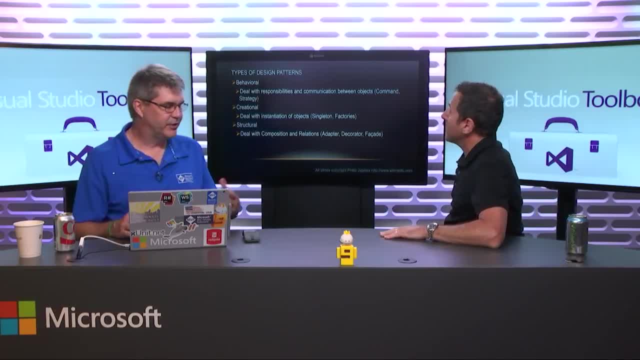 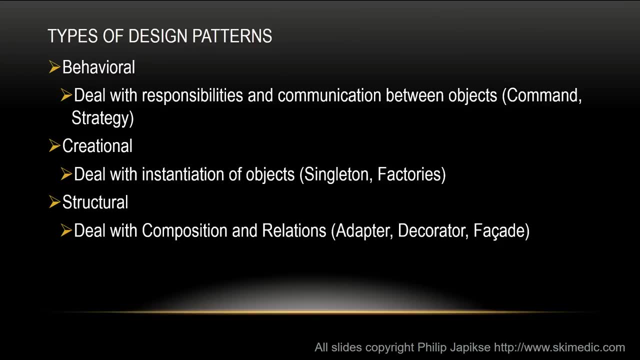 this at the beginning of the series. Sorry about that. So there's really, when you break it down academically, the gang of four who founded, really first documented all the design patterns and whatnot. There's three categories: behavioral, creational and structural. 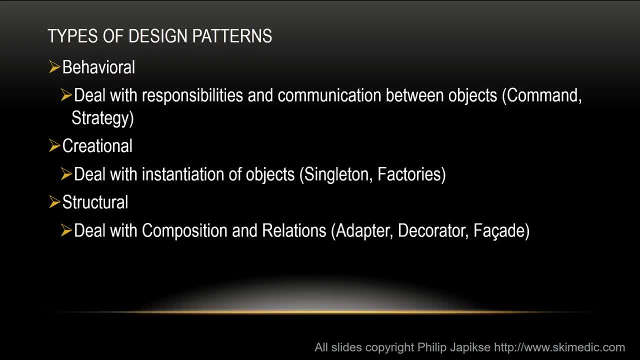 Okay, So we covered the behavioral. We didn't talk about really what that meant, but it just deals with the responsibilities and communication between objects. Okay, So, for example, the command, the strategy pattern, all those shows that we've done so far. 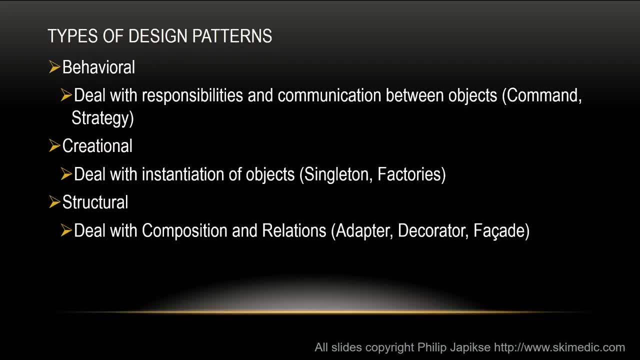 Creational, exactly like it sounds, deals with making things, Making things right. We've said several times: new is glue. We don't want to use or create something and then use it in the same method or really even the same class. 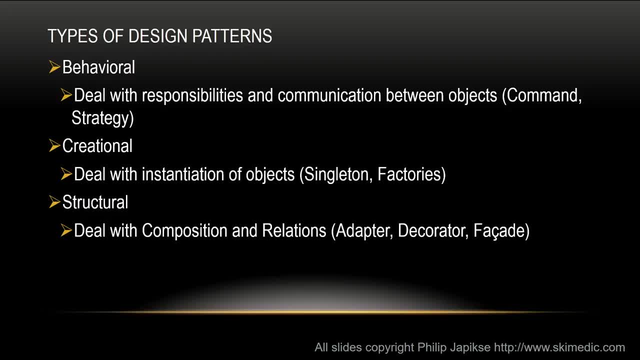 So this gives us some ways of creating things, especially when we get into the factory, so we don't have to do that. Okay, The final bucket, if you will, is structural position and relations. So we're going to talk about many of these patterns. 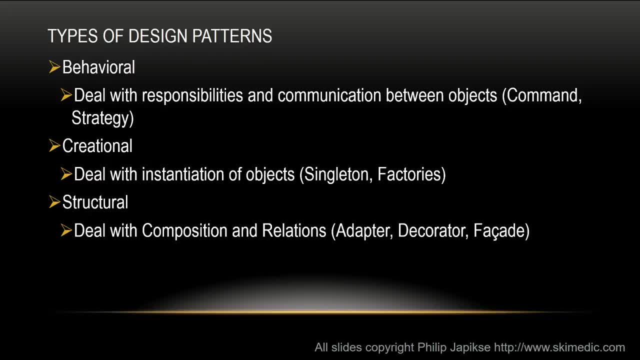 We're going to talk about all of these: the adapter, decorator and facade. Again, those are just the three main buckets. We started off with the behavioral, not because I thought they're more important, but because B comes before C. 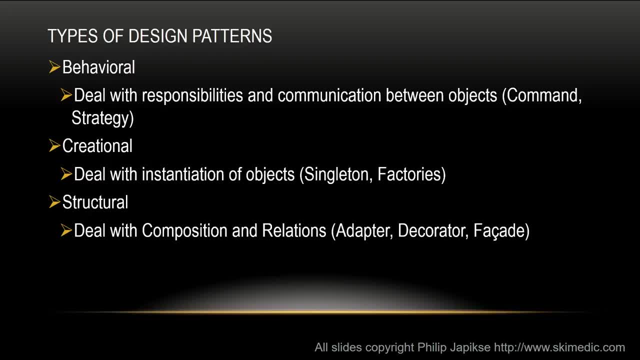 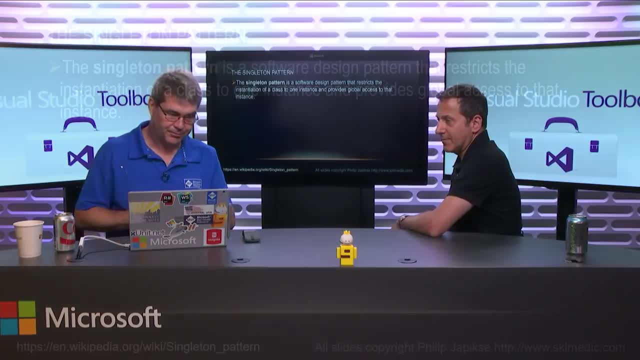 which comes before S. So that was the order that we chose for the different buckets. Okay, So today we're going to talk about the singleton pattern. Yes, we are, Okay, So the singleton pattern is used in many other patterns, right? 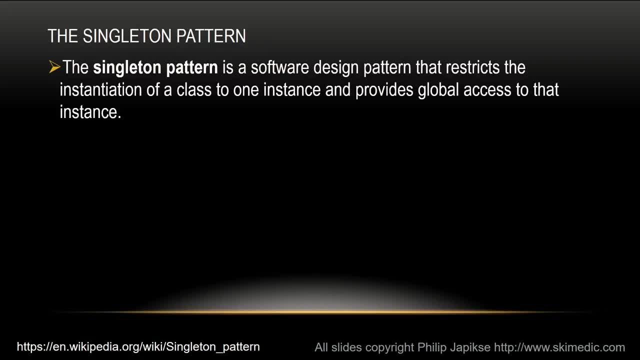 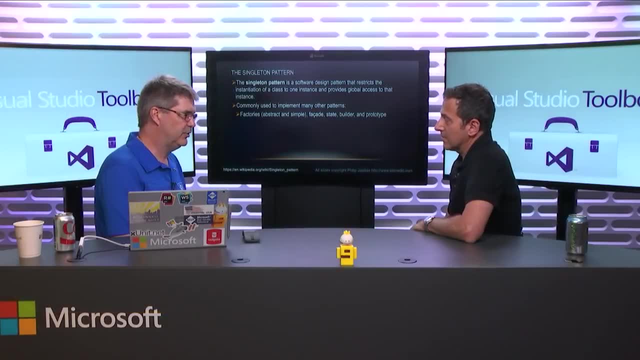 Just as the command pattern is used all over the place. we find these things blending together right. So we're going to talk about the factory patterns next, and you'll see that the single pattern a lot of times is used to create. 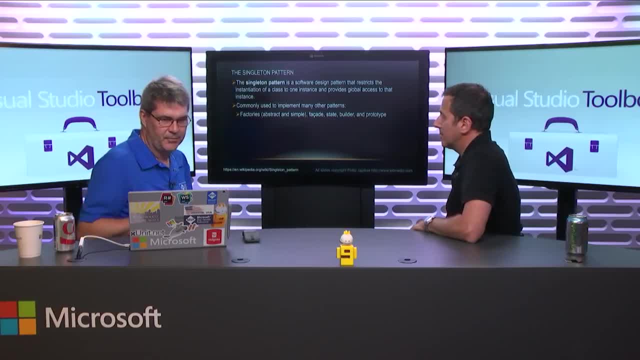 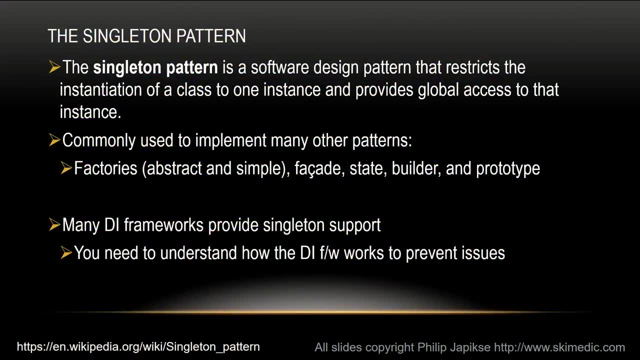 those factory objects because we only need one of them. Okay, Right, Yeah, So many DI frameworks, for example, have- Dependency injection, Sorry. Yes, dependency injection frameworks provide singleton support. Okay, Think of ASPNET Core and a dependency injection built into there. 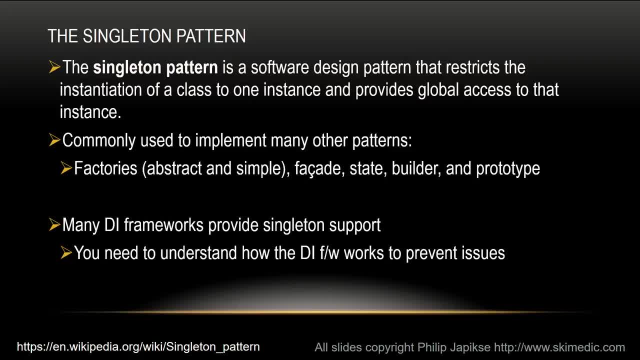 I can create something scoped at the singleton level. Okay, That means that across that entire web application, regardless of who's coming in, there's only one instance of that object. Okay, Right, So would your navigation be a singleton then in an app? 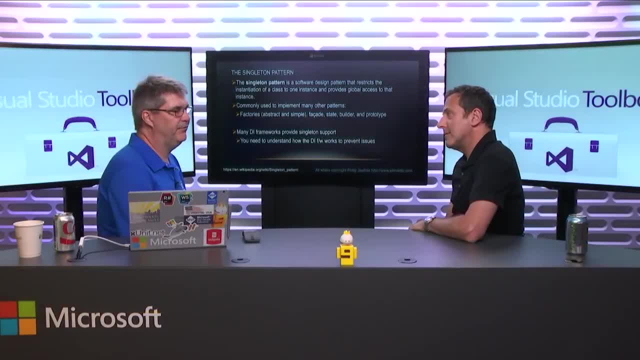 So, to be honest, I very rarely will use navigation. Navigation is a singleton. just because that can be static, right, It doesn't matter how many, All right. So let's talk about this. They're static and they're singleton and they seem roughly the same. 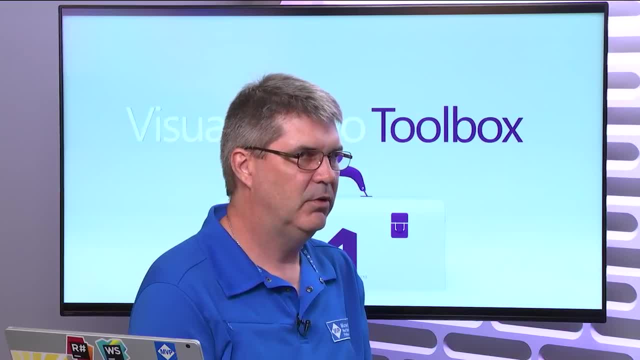 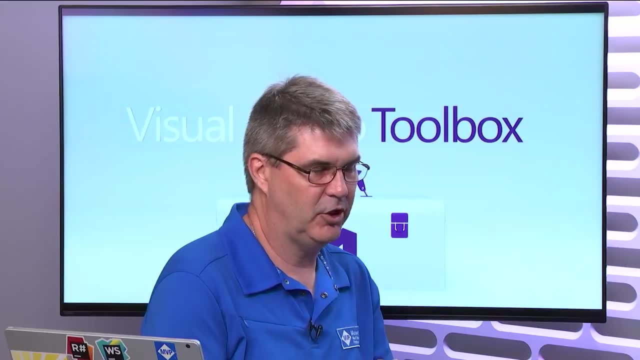 but, as is very well documented- but I will say thoroughly documented, because I've read the explanation of why they're different and I'm not a C-Sharp deep dive expert- There are some differences. Static classes are not guaranteed to be thread safe. 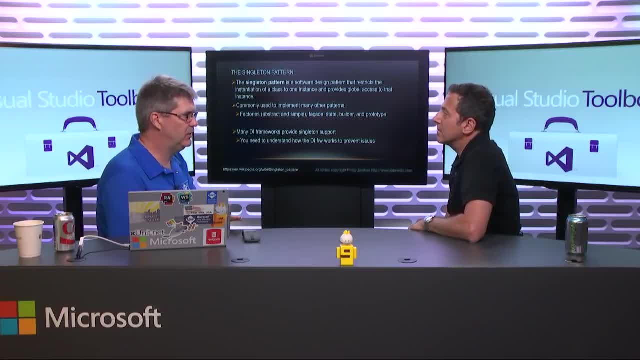 Okay, Which means you can get more than one instance in an app domain if you just make them static, Okay. People ask me why all the time I've got a link to the article. We'll put it in the show notes. It has to do with a lot of things that. 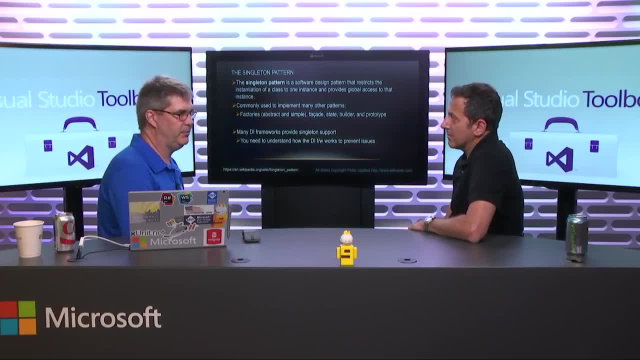 honestly, as a line of business developer, I don't go down that deep. Okay, If Microsoft says not thread safe, I say okay and I believe them. Okay, And I do it differently. All right If we're tracking something, for example. 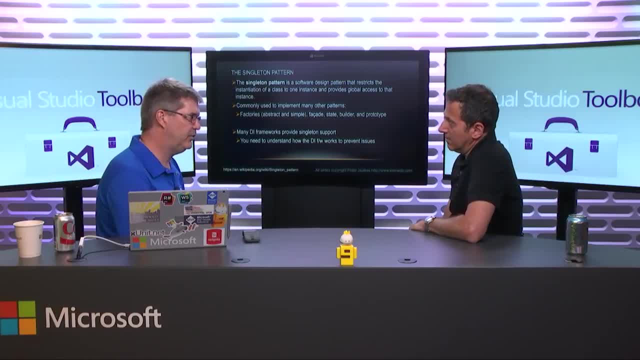 let's say you're selling ad space on your website and you have to know how many unique visitors there are. that's a good candidate for a singleton object across your entire website, because it doesn't matter if I'm hitting your website, if you're hitting your website. 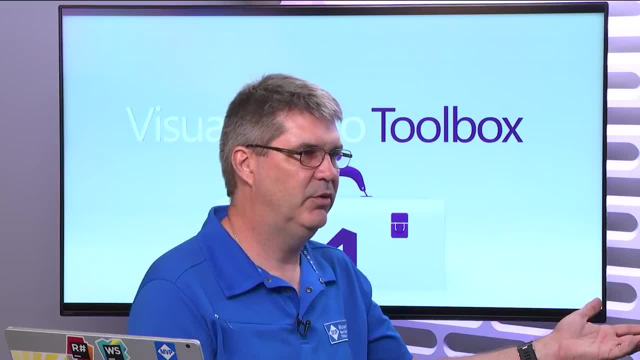 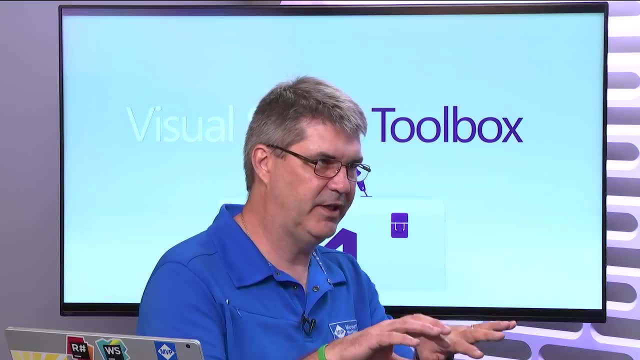 if Bill is hitting your website. you want to know how many visitors across the board? Okay. And you want to make sure you're only counting it once and that you're not splitting up multiple instances, because then you'd be losing revenue. Okay. 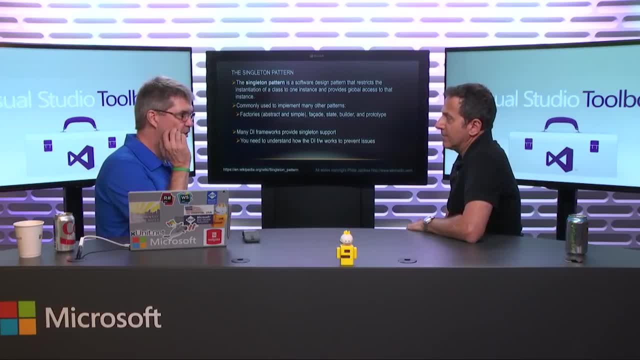 Got it Okay. One thing not to put into a singleton is, for example, a DB context from entity framework. A lot of times people think that's a good candidate for a singleton because creating a DB context is fairly expensive. I mean, there's a lot of ramp up that goes. 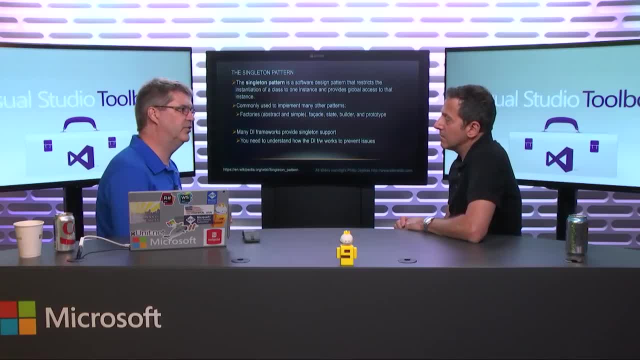 including creating connections, checking the database to make sure that it matches the schema that any framework expects. But the problem with making a singleton is the DB change tracking. So every time I pull something into entity framework I start tracking it, Right. 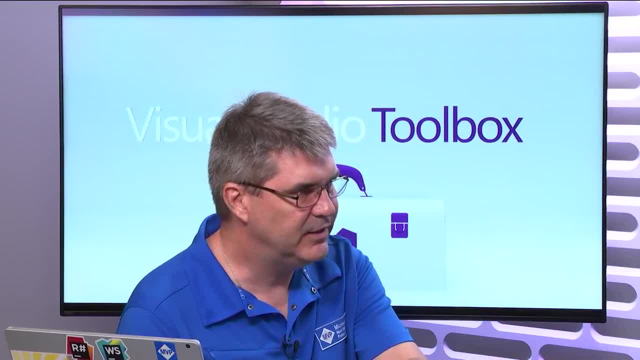 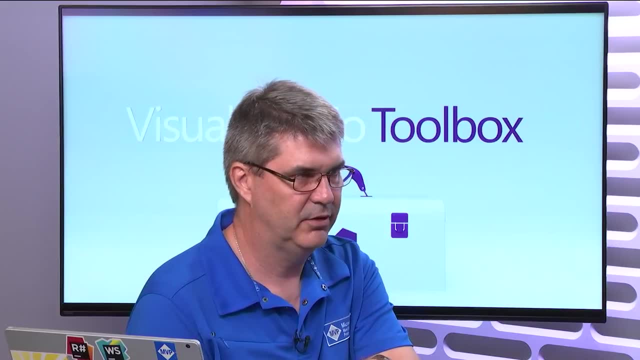 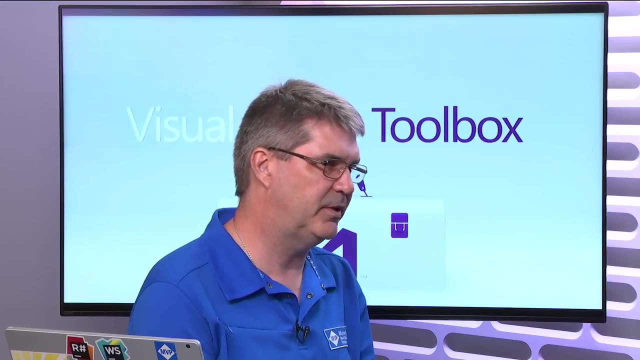 Well, you have the same instance of the DB context. Now your change tracking and my change tracking are interfering with each other, Right, And can cause really weird side effects. So, whereas it seems like a good candidate for a singleton because there's an expensive operation, 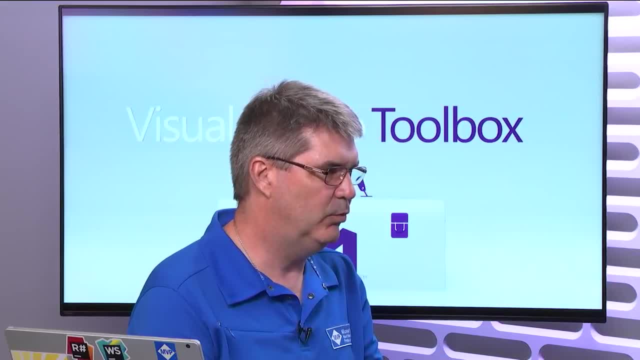 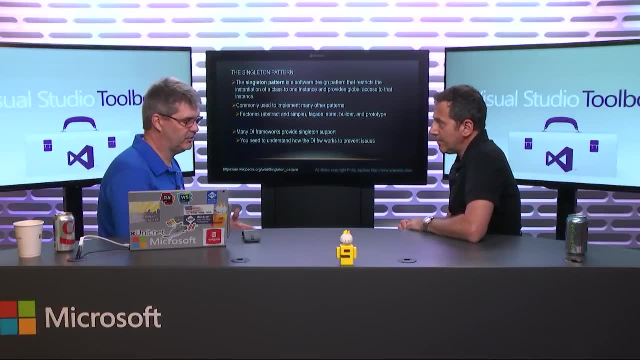 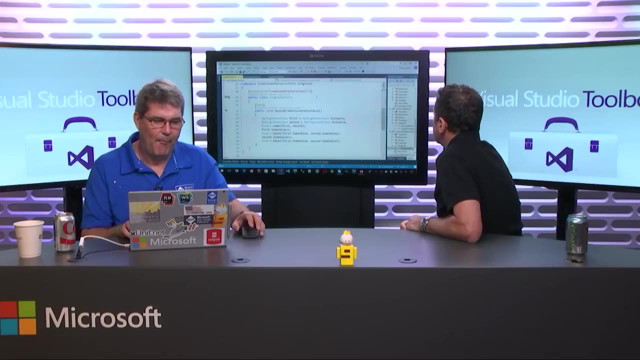 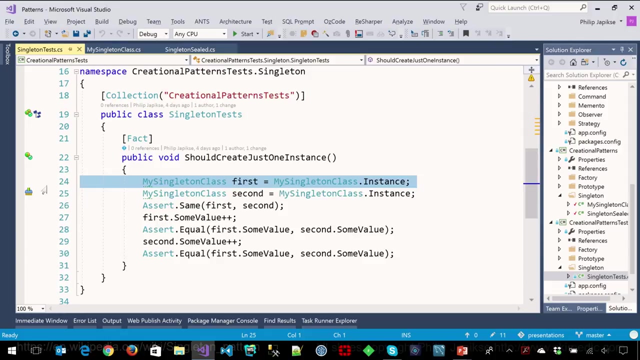 it's not Because having one globally shared instance of a context in the framework is a bad idea. Okay, So we have to really think about the use cases, Right? All right, So there are some conventions, and we did cover this pattern in the mega talk. 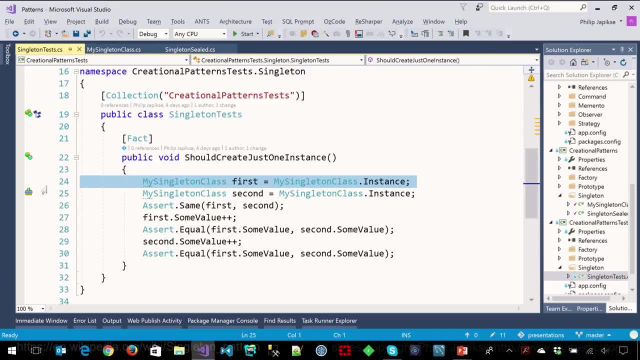 the solid design patterns from Immortals. that we did, But, like all the other patterns we covered, we really zipped right through them, Right? So this will give us a little bit more time. We'll give you a little bit more time to talk about it. 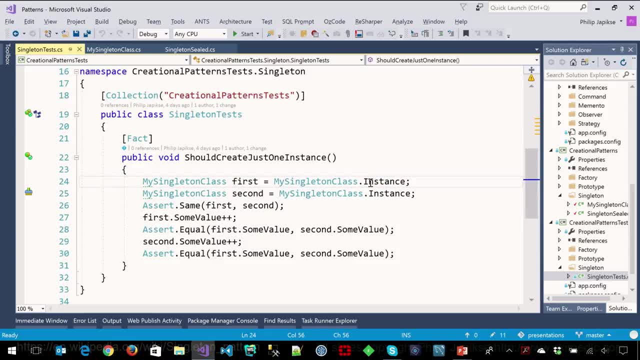 Okay And answer some questions. You can usually recognize a singleton by a static property named instance, as shown on lines 24 and 25.. There's no requirement for that. That's just the way people do it, But it's a good. 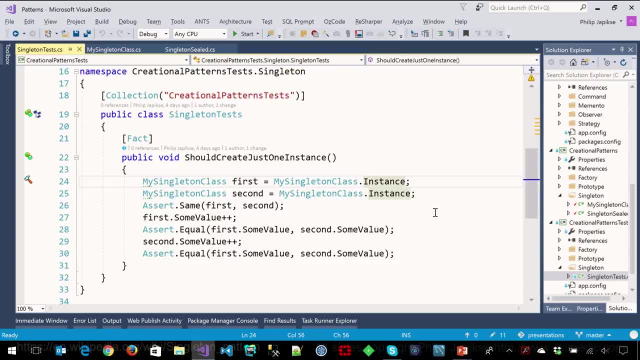 It's a good. It is a good pattern. It's a good pattern because it tells you right then and there: Yeah, And I guess I shouldn't have used pattern Practice. It's good practice, Yeah, Just like naming your interfaces with. 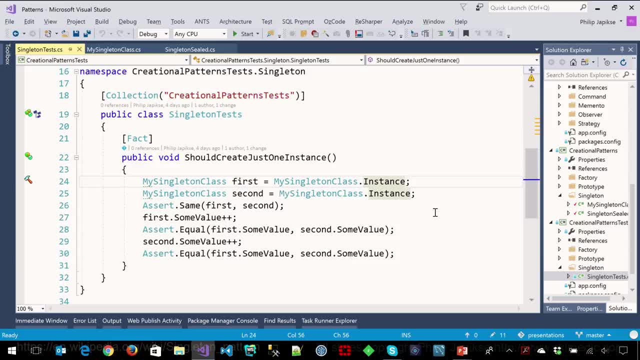 an? I? Yes, Right. So we know it's interface, Right. So I am declaring two different variables, both pointing to the instance static property of my singleton class. So it's a singleton class. It is designed to be declared once. 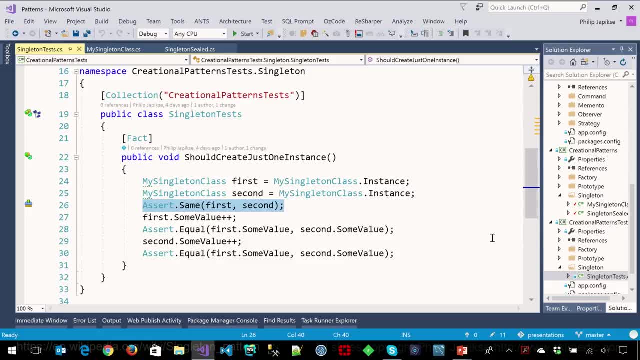 Those should be the same. Yeah, So in X unit, and this is the same for the other frameworks as well. equal and same are two different tests, Right? Equal is looking at the value. compare. Same is: are these both pointing to the same thing? 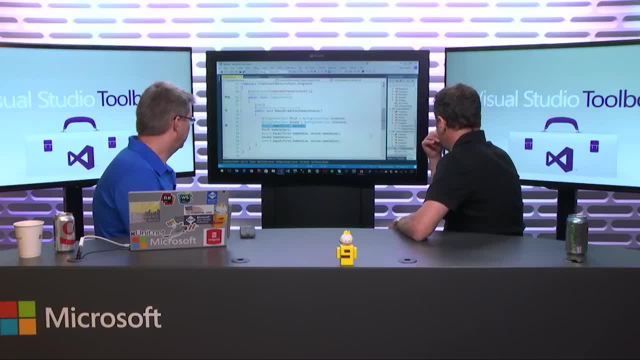 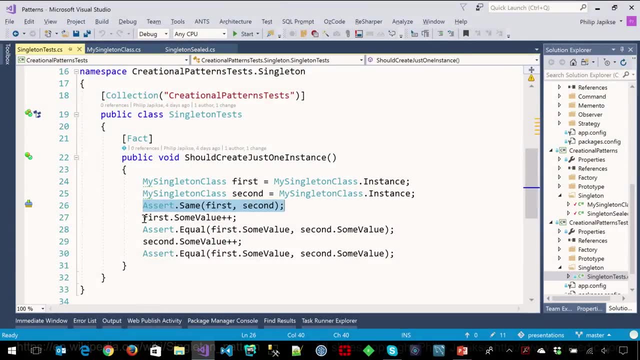 Right, Right, The same object on the heap And line 26 is just verifying that they are the exact same object. I have just an arbitrary integer property on my singleton class. I increased the value on the first variable and then I confirm that those values between the two variables are still the same. 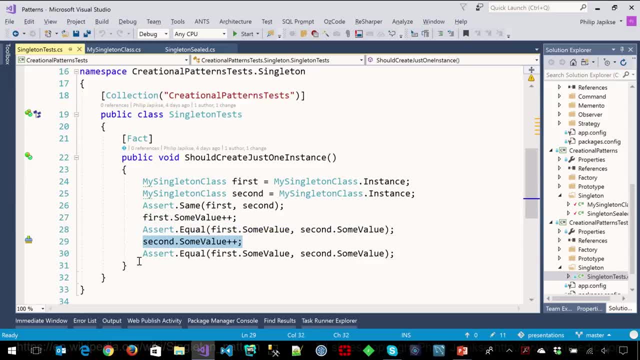 Mm-hm, And then I confirm that those values between the two variables are still the same. I increased the value on the second and I do the same. So all this test is proving is that we are, yes, indeed, pointing at exactly the same object across the entire. 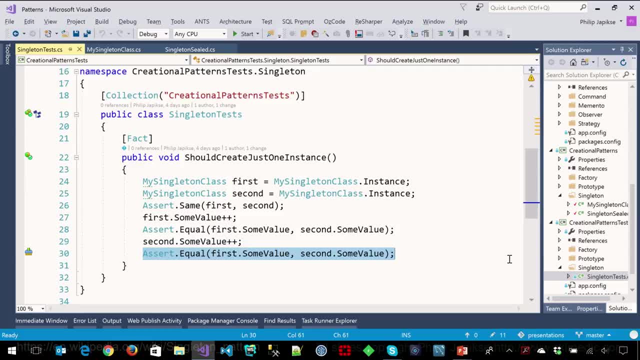 at least this unit test, right? We're not proving different users are coming in differently, Right, But we can count on it working the same way. Okay, Let's look at how to implement it, And we'll start off with my singleton class. 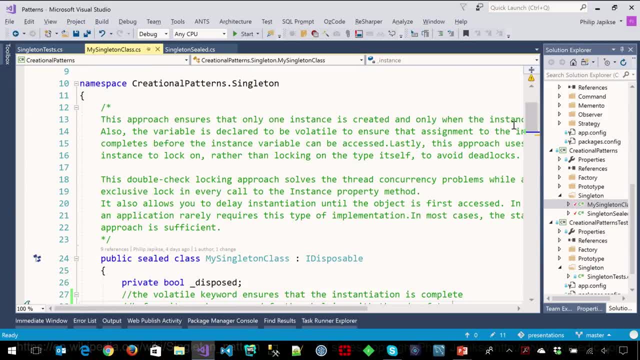 Lots of comments in here And the reason I have comments in here memory leaks- threading issues. they're very hard to prove or disprove, So I prefer to stand on the shoulders of giants. There's great documentation on MSDN about how to do singleton and how not to do singleton. 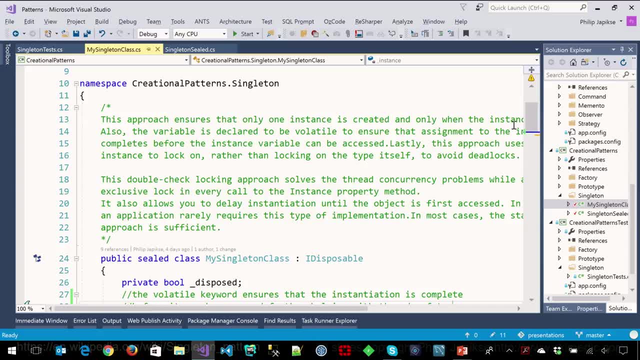 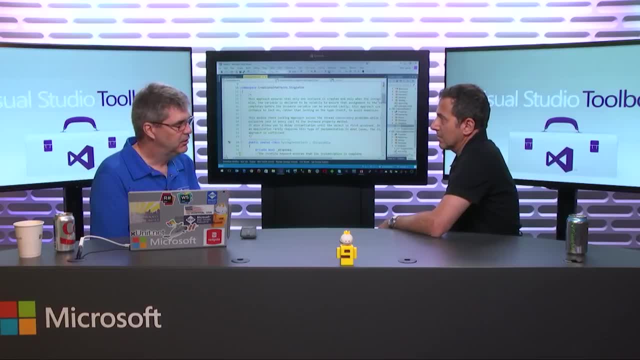 Okay, And like we were just saying before, why static doesn't work exactly the way we want it to. I'm not sure that I care. I care that it doesn't, so I know not to do it, But the comments and the links in here will point you if you are so. 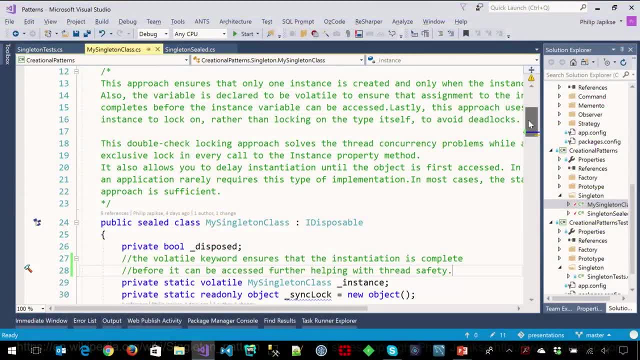 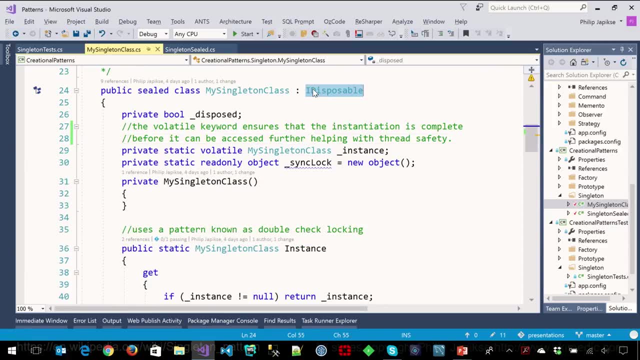 obligated to go dive down. And again, the GitHub repo will be in the show notes. We haven't said that on every episode, but it will be. iDisposable is not part of the singleton pattern, It's just a habit I like to get into to make things that might have. 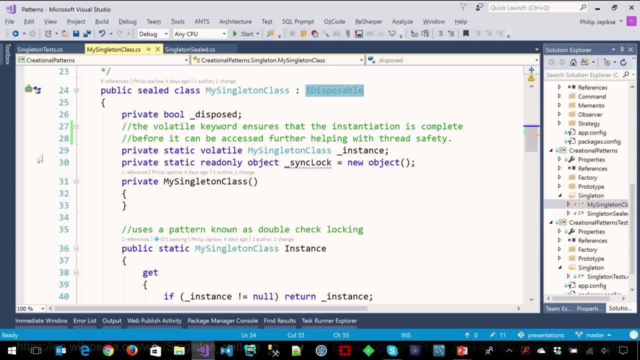 expensive resources, implement iDisposable Mm-hm. So we have a private static of my singleton class, Again, just by convention, we call it instance. We have a object. by convention, we just call sync lock. Okay, Here's the key. 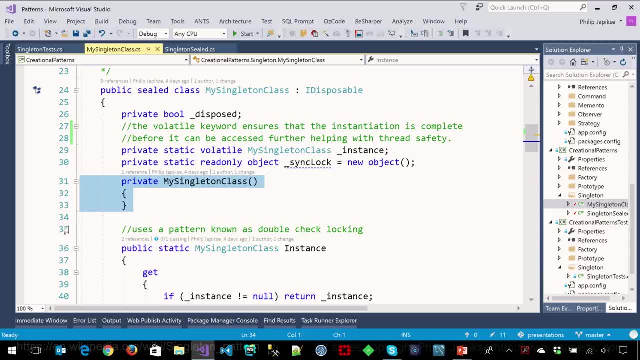 The class itself has a private constructor. Okay, So nobody outside of itself can construct a new one, Mm-hm. And we seal it to prevent anybody from deriving and changing that behavior. In general, sealing a class is probably considered a code spell. 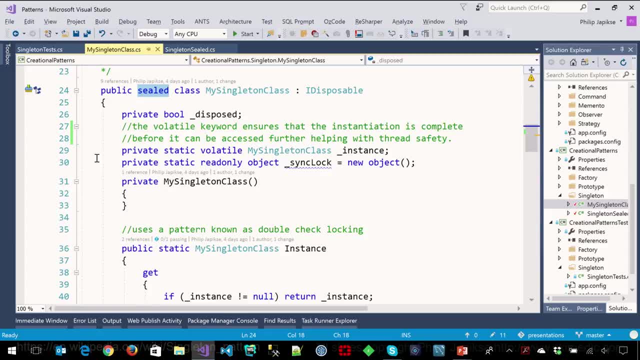 There's lots of classes in the NET framework- at least the full NET framework- that were sealed, which made unit testing very, very hard, Mm-hm. So in general, like I said, it's kind of a code spell. 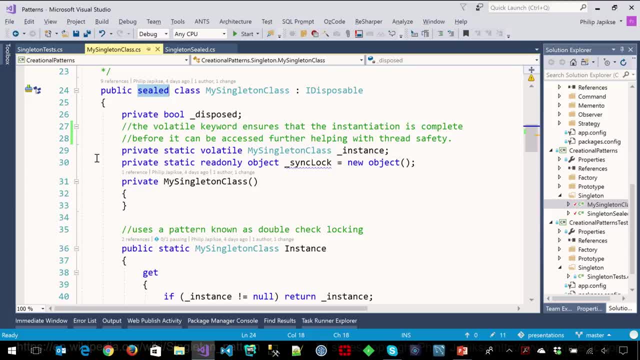 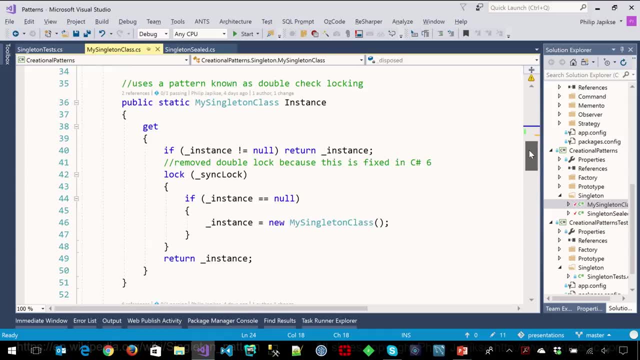 But for the singleton it's very important that you seal it Right, So nobody derives it. Nobody derives from it, thinks they have a singleton whereas they really don't. Right, Okay, And here's the magic. Here's how they make the sausage. 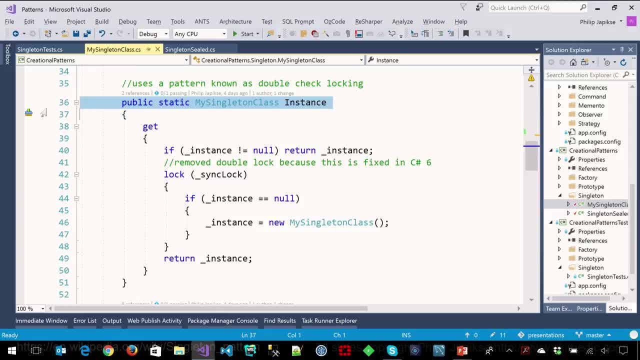 So I have a public method- sorry, public property- called instance. Again, just a convention doesn't have to be called instance. It's a good one though. So if the instance is null, this is that private variable. 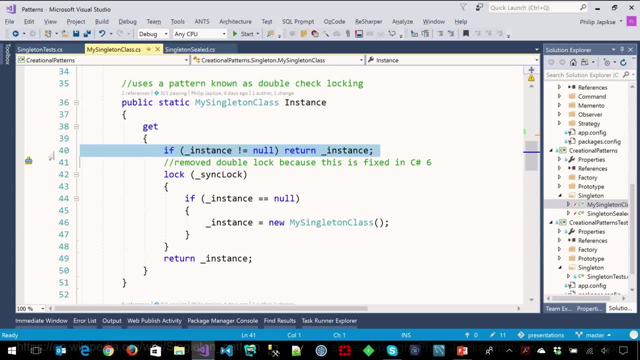 If it's not null, I go ahead and return it. I say, okay, we have one created already, Here you go, Here you go, You can use that If it's already been created, If it's already been created. 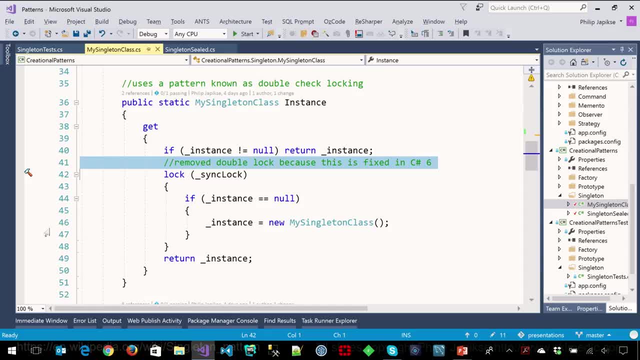 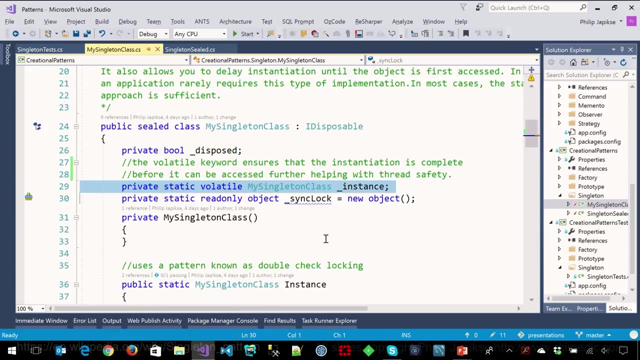 Okay, So in C sharp 6, we had a fix to static properties by using the volatile declaration. We were talking about this before we got on the air. Wait, did you just say volatile showed up in C sharp 6?? Yeah, according to my notes. 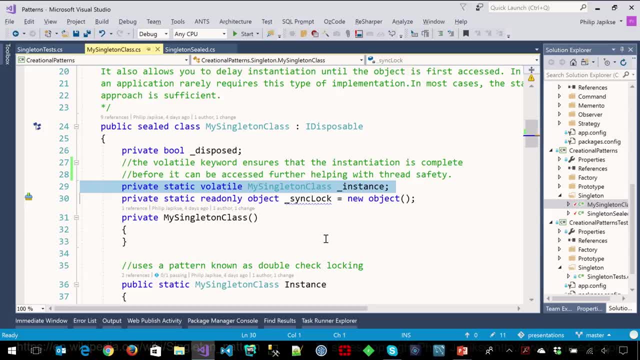 Oh, okay, We were talking about this before for the viewers. I hope you liked the little banter that Robert and I do on the shows. It seems to have gone well in the past. I couldn't remember what version volatile showed up in. 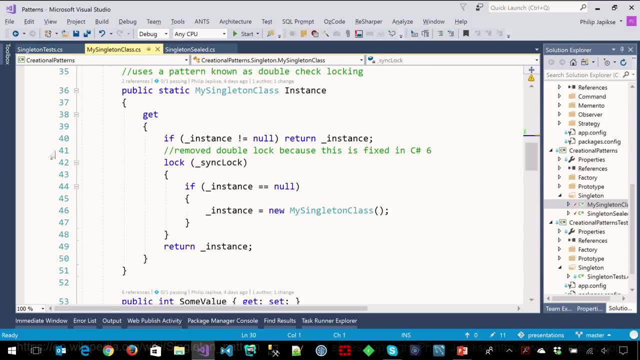 So it was in 6.. And then I go right down here and it says: remove double lock because this is fixed in C sharp 6.. Okay, Now volatile might have been there before C sharp 6, but it didn't work right. 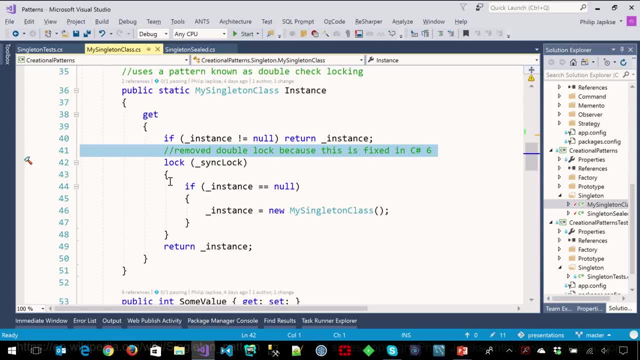 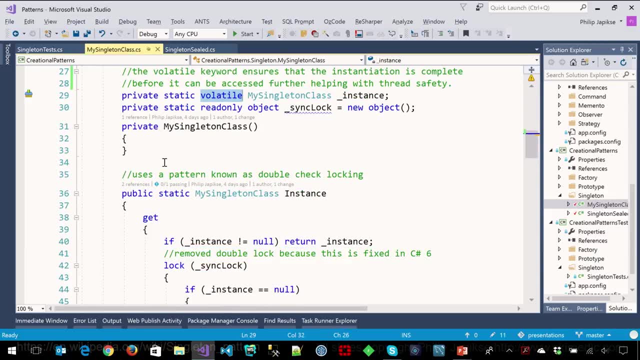 Ah, okay, So we're going to go with that because I'm not going to take the time, while we're recording, to research when it came. Yeah, it doesn't really matter. There is a volatile key. Yeah, The volatile keyword. 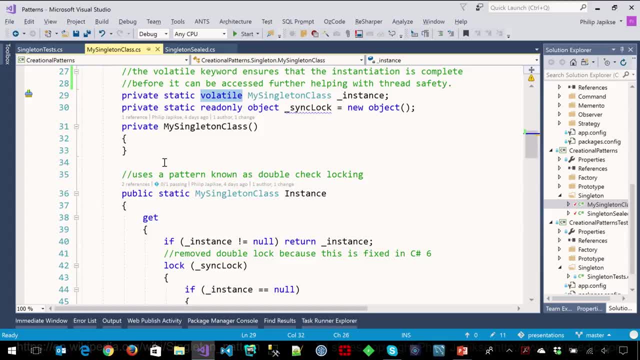 The volatile keyword: Yes, And in C sharp 6 and later, it works as expected. Okay, The volatile keyword, as the comment declares, ensures that the instantiation is complete before it can be accessed. further helping with red safety. Okay, Now how does this play into the whole mix? 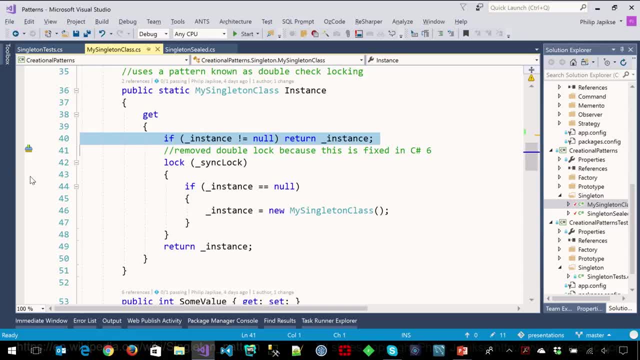 Let's go back to our instance Right here. we're not locking, We're not doing anything. We're saying: if the instance is created, here you go, Have at it. Mm-hmm, Line 42 is locking this block. 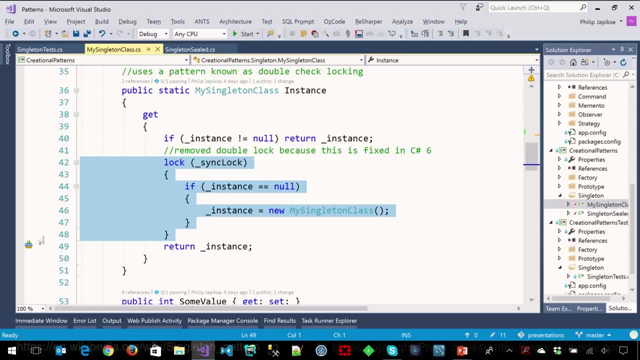 This means it's only single-threaded. We don't lock outside of line 42 because we want them to be able to get to line 40, multi-threaded, If the instance is already created. we don't want to hold them up with arbitrary single-threadedness. 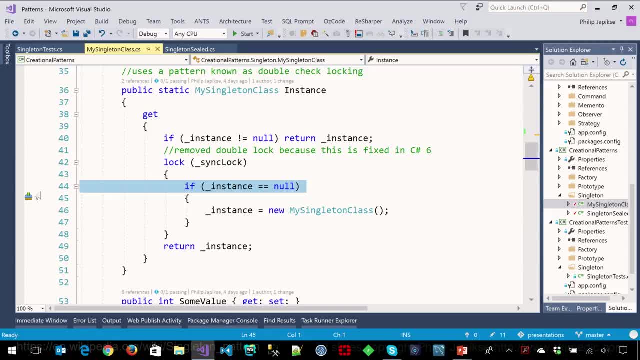 Prior to the volatile fix in C sharp 6, we would have to add another lock on line 46.. We would have to add another lock on line 46 to make sure that the instance was created. But if we back up and look at line 44, if the instance is null, right, so even if I 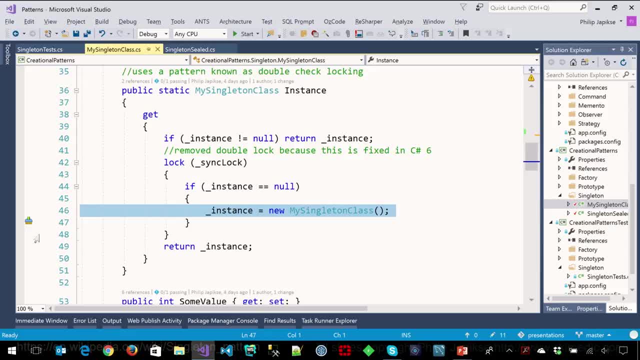 have multiple things coming through and hitting line 42, only one of them gets through. Okay, Instance is null. It goes down, creates a new instance of the singleton class. Mm-hmm, We've got the volatile keyword on it, which then means that it won't move on until. 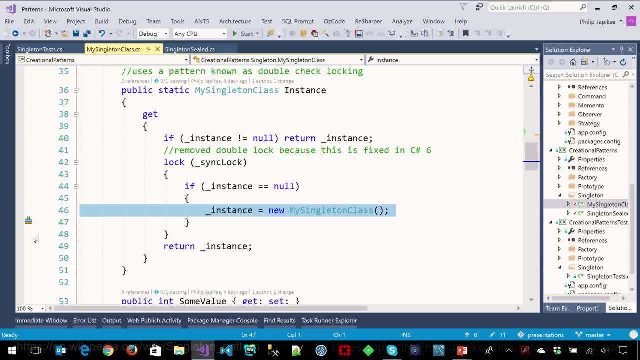 it's completely instantiated, Okay, And then on line 49, we return the instance. Yep, When we get to line 49, the next request gets released by the lock. comes in, sees that instance is not null, pops right out, returns the instance. 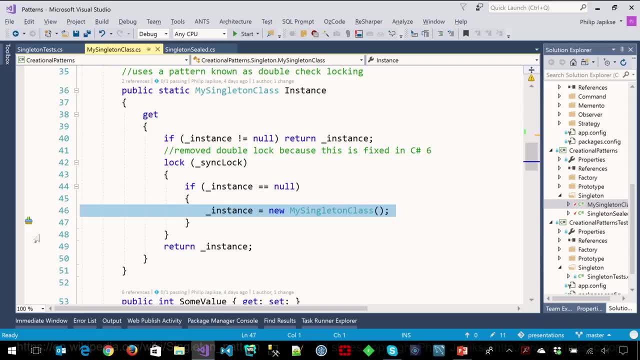 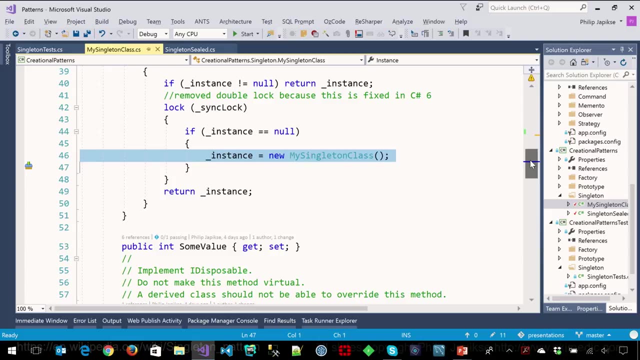 Right, So the only ones that are held up are the ones that came in at the same time or before the instance was completely instantiated. Okay, And then the rest of that is just a class. I have values, I have properties, I can have methods. 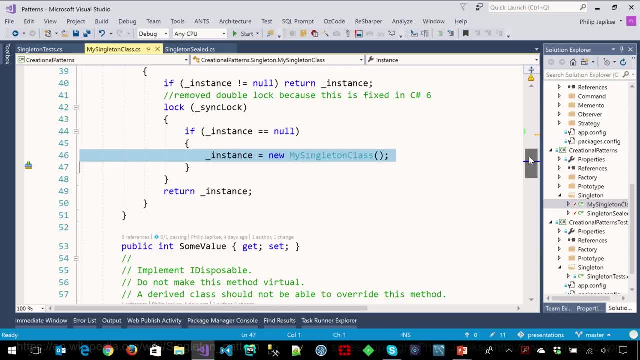 I can do everything else. It's good practice to implement IDisposable. That's not really a design pattern, It's just something we should do in C-Sharp to clean up after ourselves. Mm-hmm, So we can take a moment to talk about that. 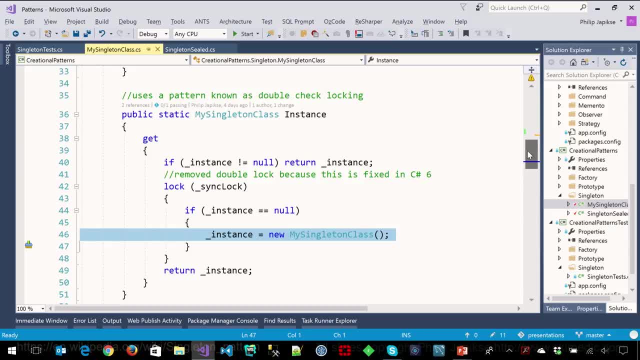 When something is marked for garbage collection, it's been disposed And I'm sure you've had shows on garbage collection and how all that works, So I'm not going to go into deep details about that. Mm-hmm, I'm sure there have been shows on garbage collection. 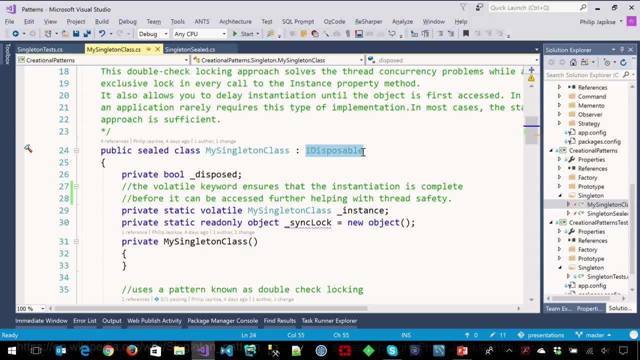 Okay, And I'm sure you've had shows on garbage collection and how all that works, So I'm not going to go into deep details about that. Mm-hmm, I'm sure there have been shows on garbage collection, Okay, So what we want to do is, if we know that we're done with a particular resource we want, 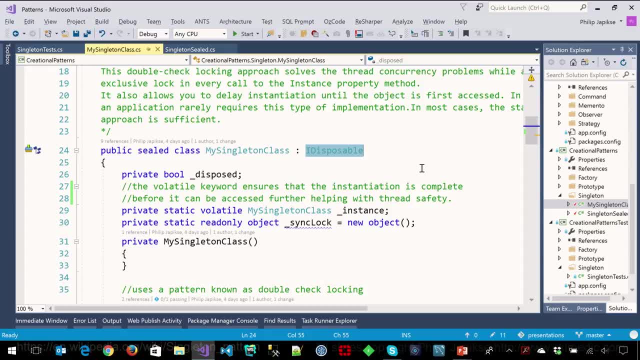 to go ahead and dispose of it so that the garbage collection happens earlier. Mm-hmm Right, There's different generations of garbage collection and lots of magic behind the scenes as to when NET clears memory. But we want to be the good citizen and recycle as soon as possible. 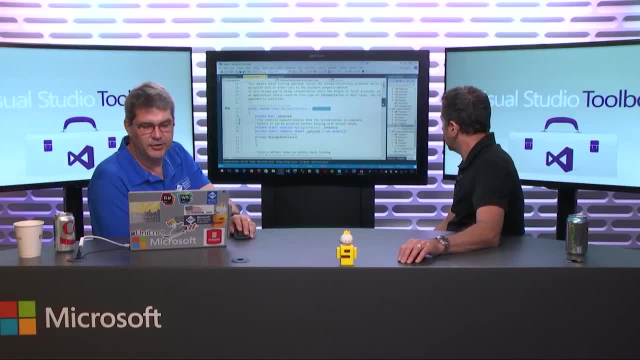 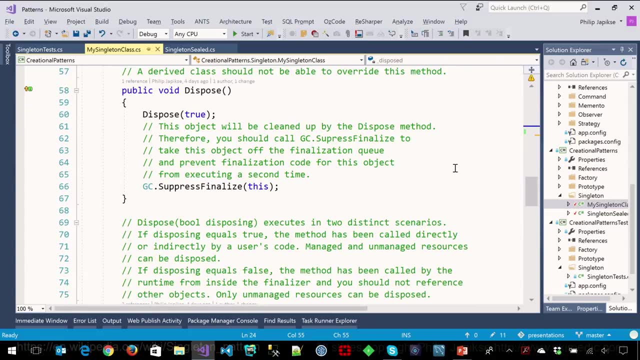 Right, Mm-hmm, Put it in the blue bin. We do that with the IDisposable so that we can call dispose And in the dispose method, again plenty of comments. here again, not a design pattern, but something that's good to do. 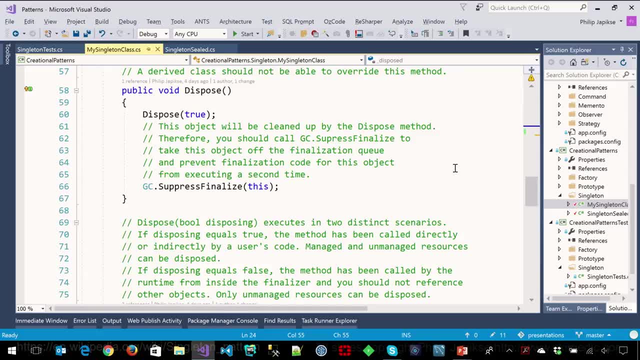 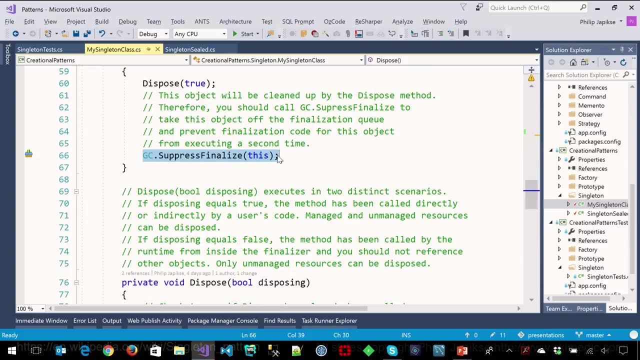 Okay, Right, So I just figured. since this is a short episode on the singleton, we'll fill it with some other good information for cleaner code Sure. So if dispose is called, then we tell the garbage collector: nope, we've already been. 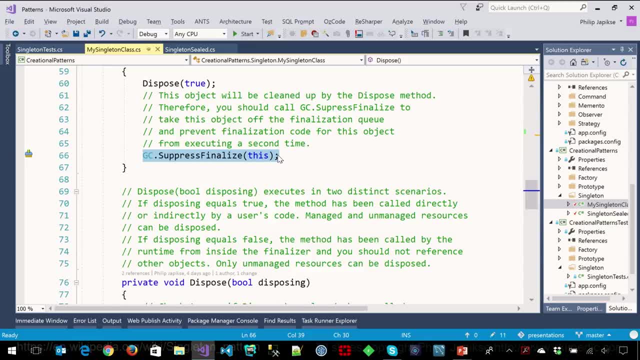 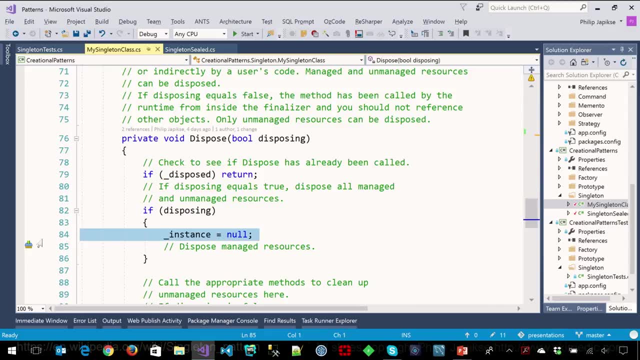 disposed. please don't call us again, Okay, And then here in the dispose method, anything that is expensive, we would just set to null. So if we've got in, you know, full NET framework, if we've got pointers or if we've got you, 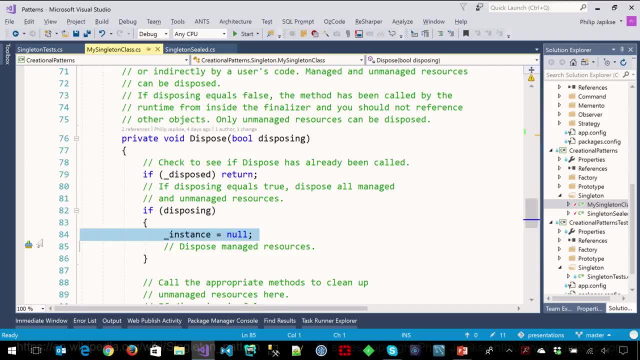 know connections to the database, things like that, we would release them. Okay, So there's not a whole lot to talk about that either. If you follow the instructions that are in the comments of the code, it all works out for you magically. 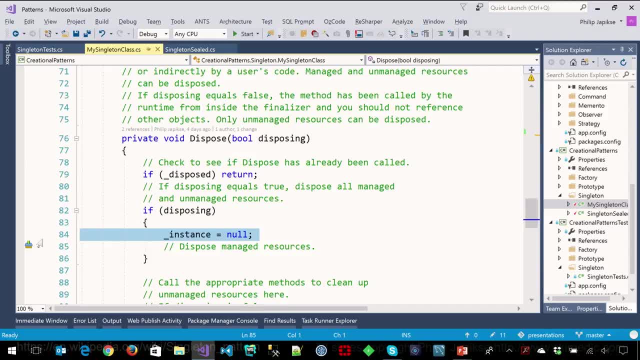 Right, awesome. So again, singleton is when you have a class and you need to ensure that it only gets instantiated or created once, Yes, And that the entire global world, you know, is going to be able to see that Right. 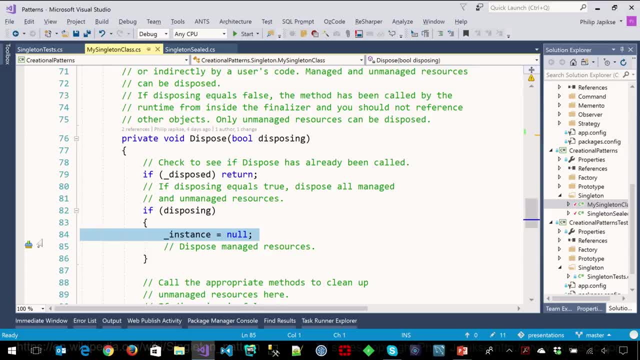